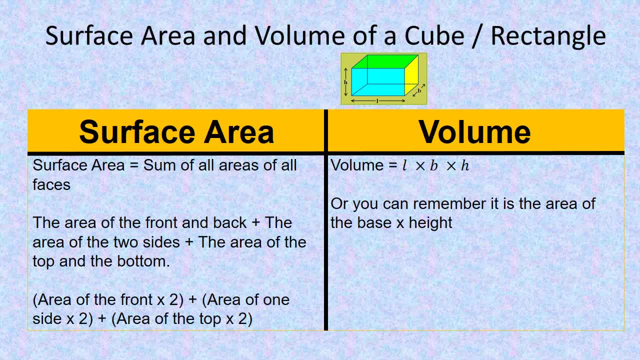 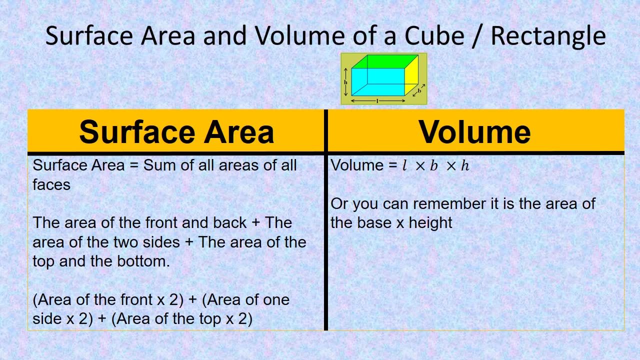 Rectangles. Now, if you look at those, two of them are actually the same, or three of them are actually doubled up. The front and the back is the same. the two sides have the same area, as well as the top and the bottom have the same area. So you can just work out the top and double it front and 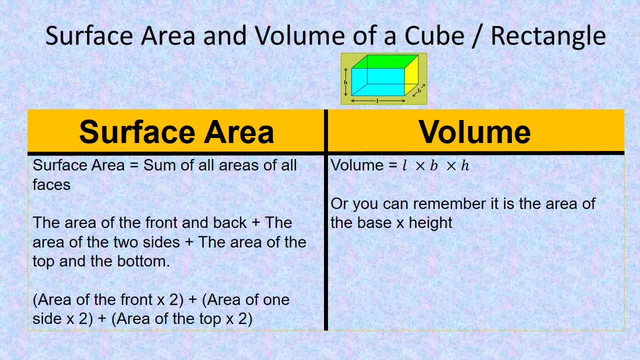 double it and the side and double it. Okay, but we'll have a closer look just now. So, just to recap, the area of the, you're going to say the area of the top and the bottom. So you're going to say the surface area is the sum of all the areas, of all the faces, and there's six of them. Okay, sometimes. 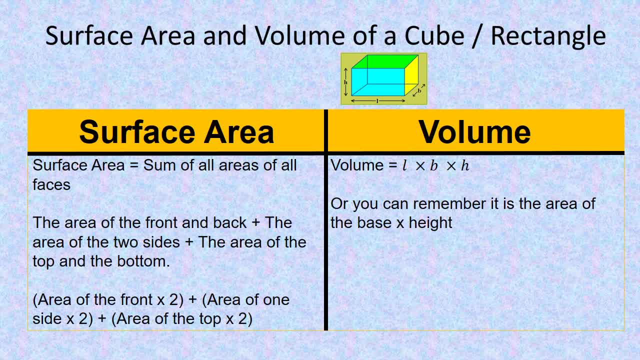 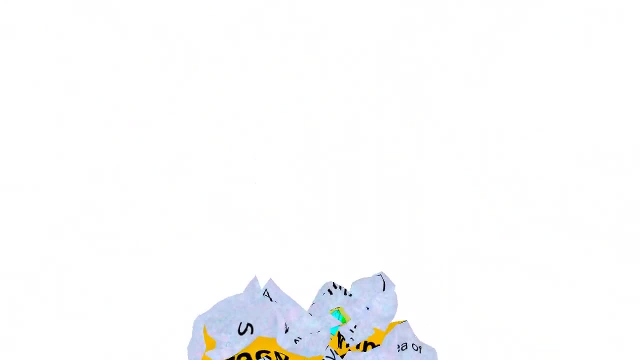 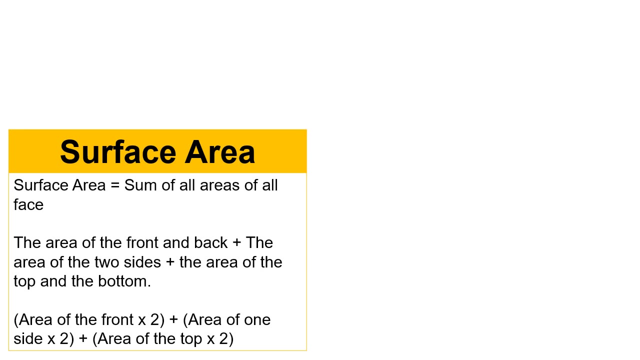 when it's an open top, you won't include the top of that area, but that's for another day. Okay then, the volume is length times breadth times height. Easy peasy, so so easy, Okay. so there, just for us to refer to, is the surface area- again A reminder- the area of the front and back plus the area of 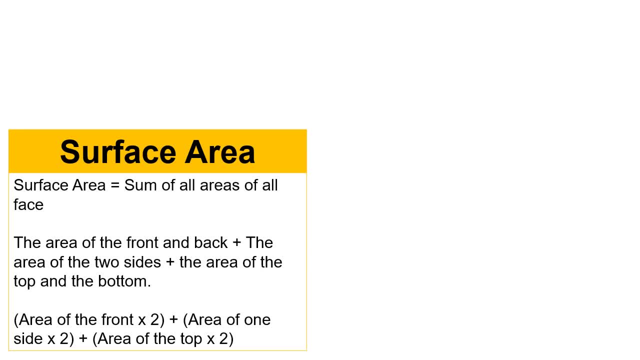 the two sides, plus the area of the top and the bottom, and the rectangular prism is made up. all the faces are made up out of rectangles, So let's have a look at this one. It's got a height of three meters, a length of five meters and a breadth of three meters. So just for, 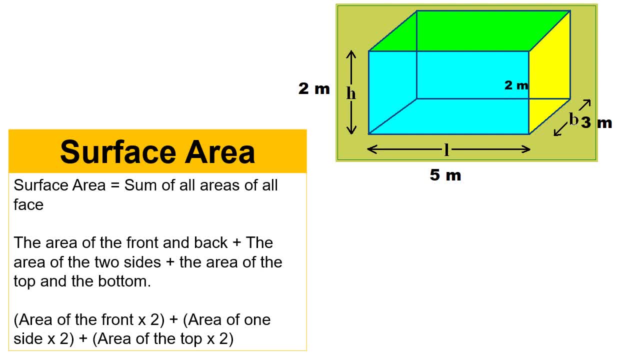 referring or to check my sides very carefully. I'm going to place in all the heights, So can you see? it's all the lines going straight up. that runs vertically. Those are two meters, So I could have placed it there, the back as well. I see I've missed that one, but all of those are two meters. Then the same with the. 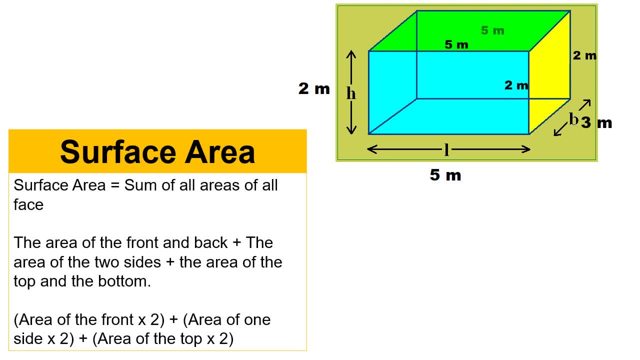 five meters. Those are all the lines that run horizontally, Okay, and I'm inserting them just as frame of reference. And then the same with the slanted, slanting sides. Those are all three meters. Okay, that will help you, especially when you look for. 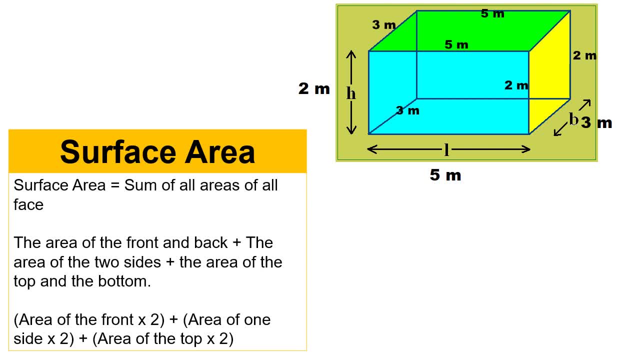 the length of the breadth, let's say of the side, or the length and the breadth of the top. It just helps you very closely or very easily to see the length and the breadth so that you don't work with the wrong distance. Okay, so surface area, let's work it out So for the front and 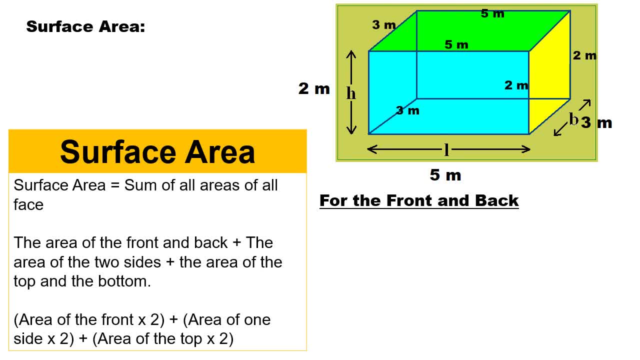 the back. do you see? the front and the back is the same. So I'm going to work out the front and the back. So for the front is the blue colored rectangle and the length times the breadth. Can you see that? it's five times two? Okay, length times breadth, But I have to times it by two. I have to. 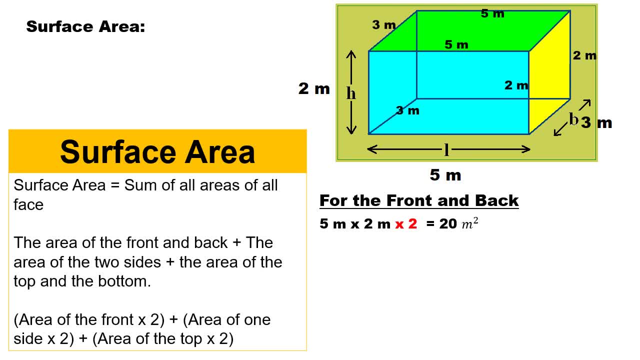 double it up for the back as well. So five times two is ten. Ten times two is 20 meters squared. Okay, let's keep that answer Then for the two sides. I'm only going to work out one side and then double it up So quickly. 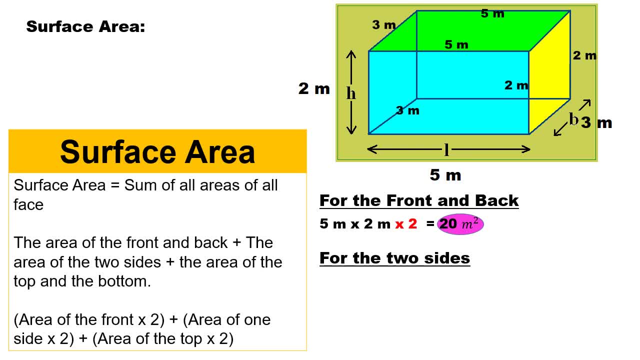 take half, take a few two seconds to quickly see what is the length and the breadth of the side which is the yellow rectangle. Okay, could you see that it's three times two? Well done, if you did So. three times two, and I'm going to double up again: Three times two is six times two gives. 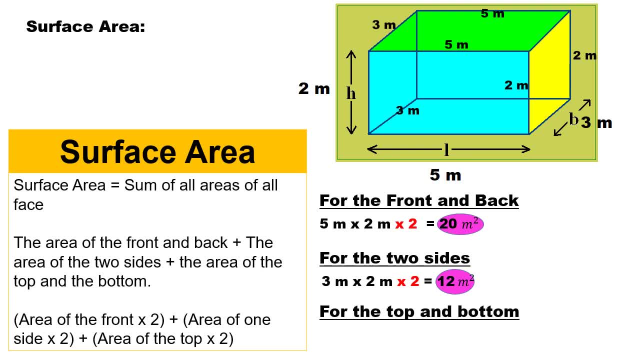 you twelve meters squared. I keep my answer Then for the top and the bottom. Okay, so the bottom, I'm going to only work out the top and I'm going to double it up because the top and the bottom is the same area. Can you see the length in the breath? Well done, Five times three. 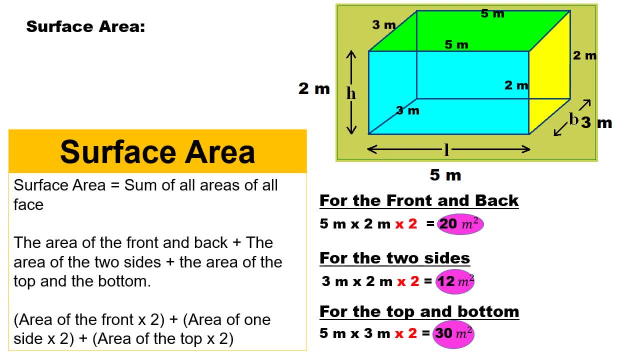 is 15 times two, because I'm doubling up. Please, you will. in the test, I promise you you're going to forget two times by two. Just remember that. Okay, And then you've got all the areas of the six different sides, or the six sides. So how do you find the total surface area? You add all your. 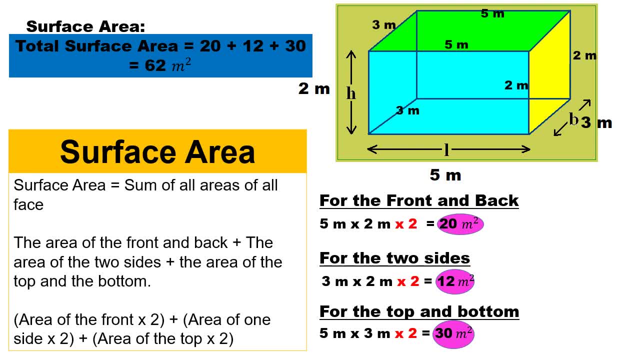 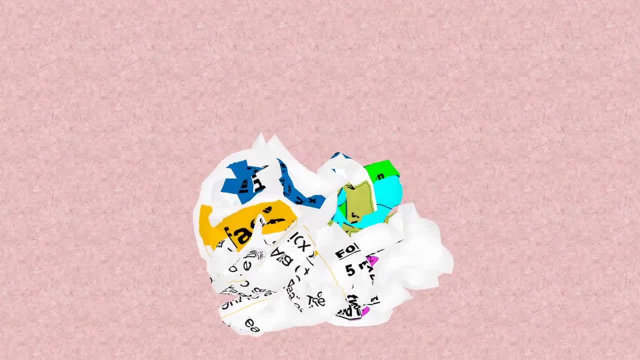 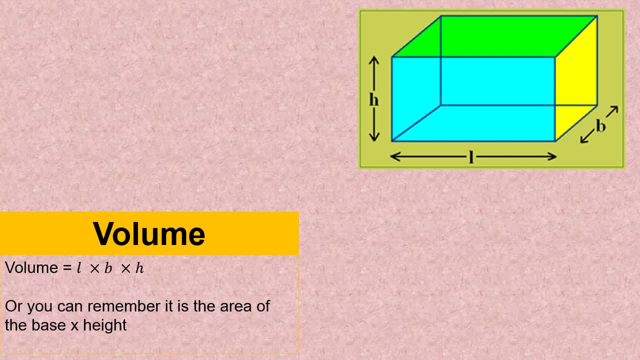 answers together. Okay, You add them back together. 20 plus 12 plus 30 gives you 62 meters squared. All right, And now for the volume, which is the easy one. Again, if you have a rectangular prism, the length is five, the height is two. 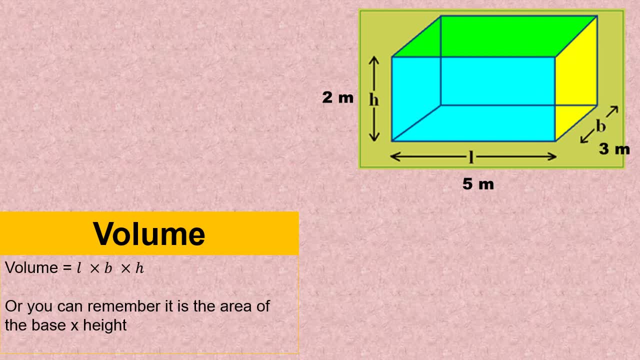 and the breadth is three. Okay, And very easy. The volume is length times breadth times height, So five times three times two. Okay, Insert that And that should give you 30 people. Very important. your units Meters cubed, Because we're working with the volume. it is meters cubed, All right. 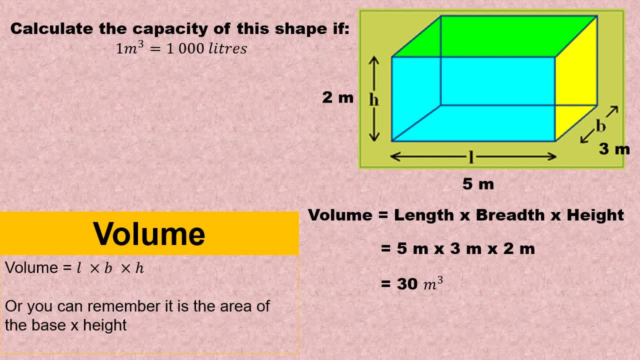 Then, just as an add-on extra is, I can actually ask you what is the capacity of the shape If one meters cubed is 1,000 liters. Okay, One meters cubed is 1,000 liters, How would you work? 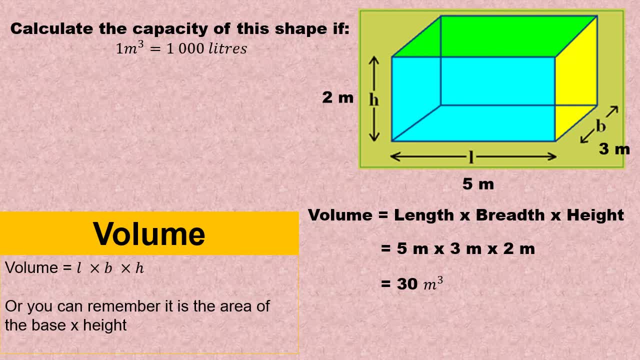 that out. An easy way perhaps to say: well, if one meters cubed is 1,000, then 30 would be 30 times that. So 30 times 1,000 is 30,000 liters, And that would be correct. Another way is- I also refer to it- 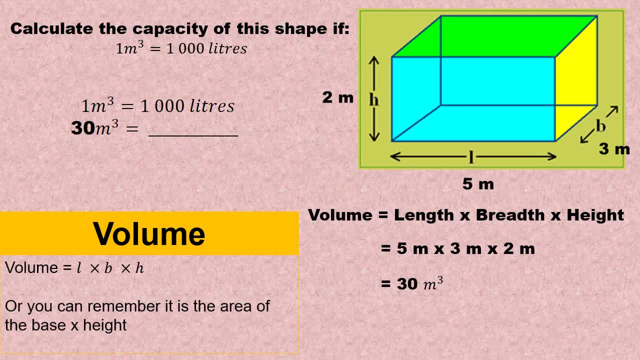 as the pirate method is, you write down what you have, And then you write down what you have And you write down what you want. So what I have, what I know, the statistic is: one meters cubed is 1,000 liters. But I don't want a meters cubed, I want 30 meters cubed. So always take from the 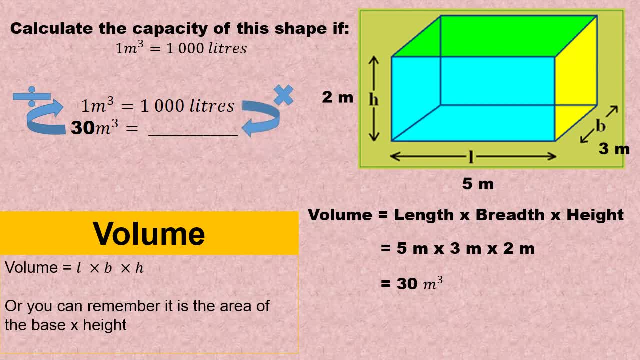 bottom, divide up and times down to get your answer. So 30 divided by one times 1,000 will give you 30,000 liters. Okay, So if that was a little swimming pool, that um amount of the the capacity that it can hold is 30,000 liters of water. 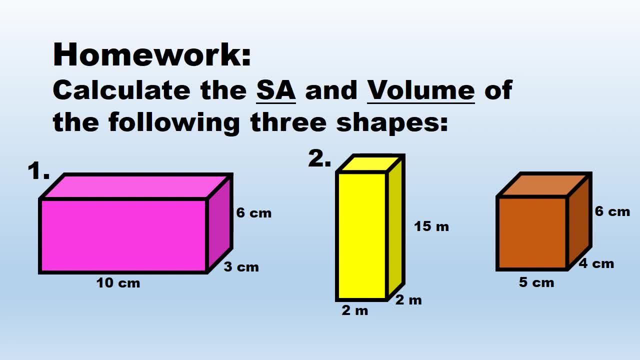 And there's your homework, Um. this will also be found on your um to-do list, So please have a look at number one, two and three. Calculate the surface area and the volume of these three different shapes. Have a great day, Great day. Thanks, babe, Bye.